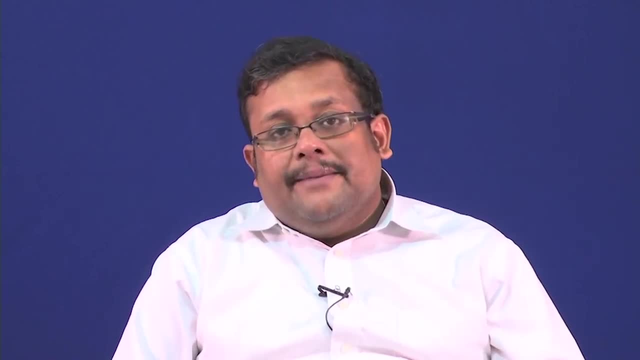 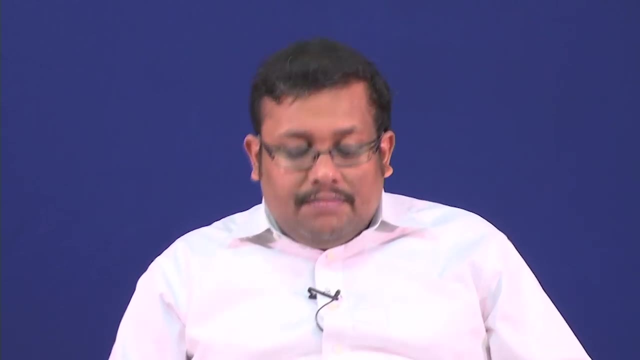 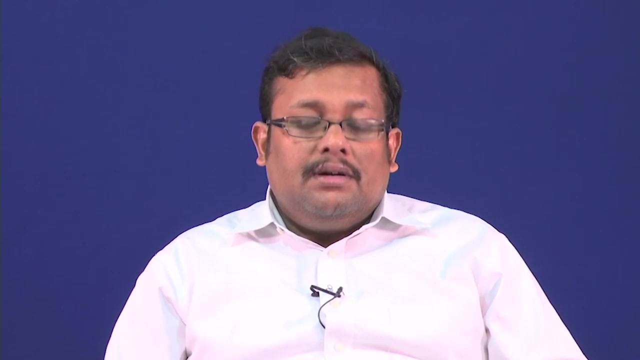 cover layers, soil and then soil temperature and different related numerical problems. So in this first lecture we will start the flow of liquid water into the soil and we will try to finish that. So we will finish it and this flow of liquid water into the soil, and then we will go to 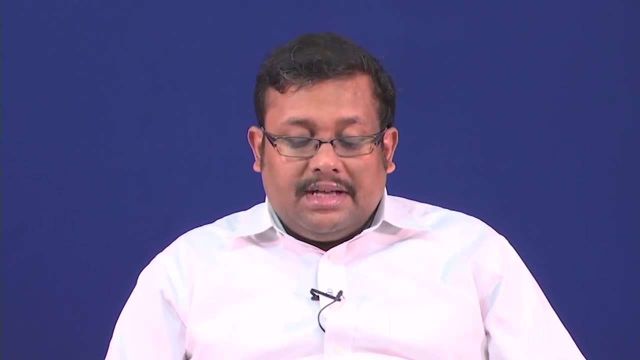 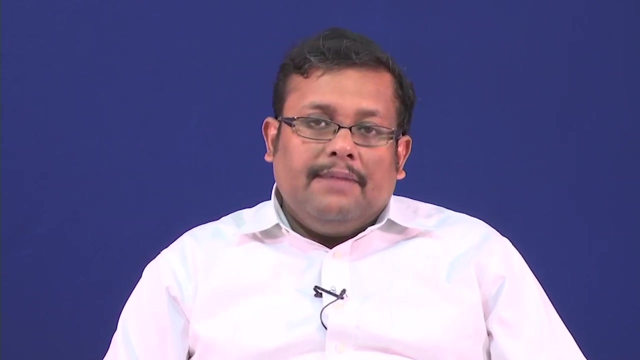 the next topic of soil water. that is different content, different, you know, gravitational water, what is the plant available water? and then what is bulb, what is fill capacity, what is permanent wilting point? we will cover in the next lecture also. So let us start with this flow. 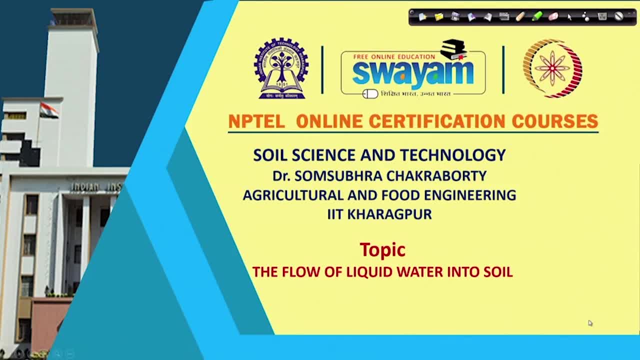 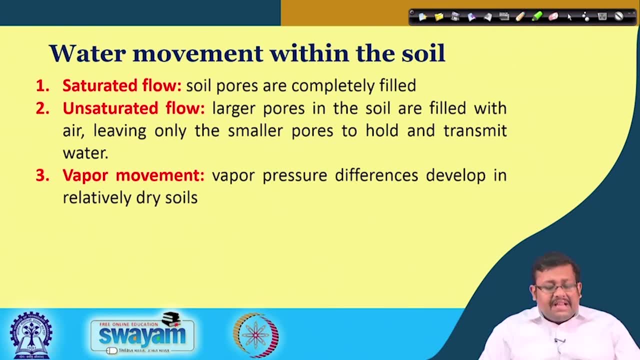 So let us start with this flow of liquid water into the soil and in this lecture we will be basically covering different saturated and unsaturated flow and vapor movement within the soil. So- and there are different aspects, So water movement within the soil can be. 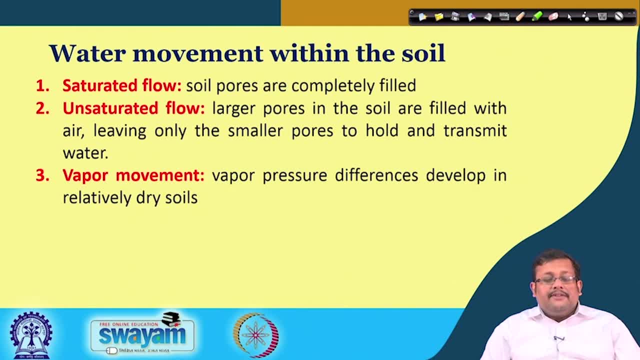 of three types: one, the first one, is saturated flow, the second one is unsaturated flow and the third one is vapor movement. Now, in case of saturated flow, the major characteristics of saturated flow is soil pores are basically, you know, completely filled. So saturated flow occurs when soil pores 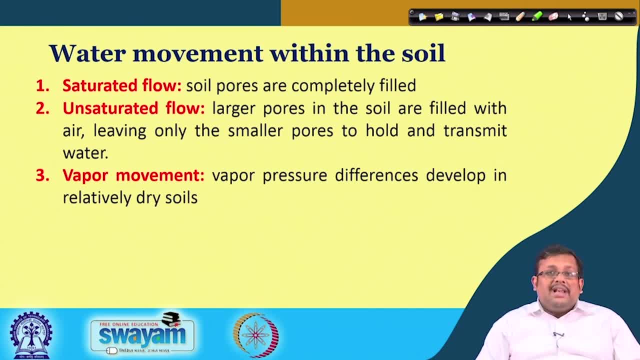 are completely filled. unsaturated flow occurs when larger pores in the soils are filled with air, leaving only the smaller pores to hold and transmit water. So this is the difference between saturated flow and unsaturated flow. And finally, another type of movement is called vapour movement and vapour movement basically. 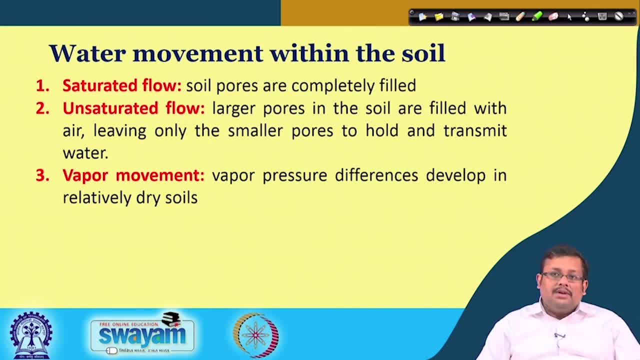 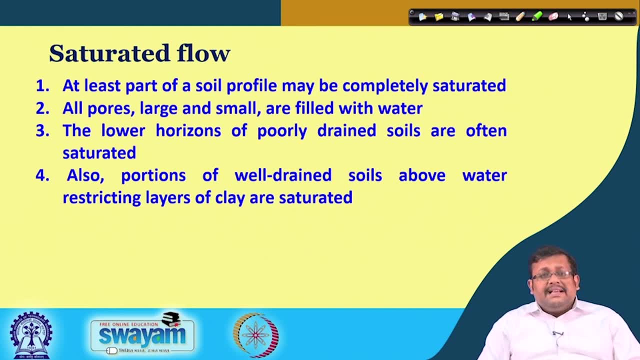 occurs due to vapour pressure differences develop in relatively dry soil. So let us start with the saturated flow. So saturated flow is basically, at least part of the soil profile may be completely saturated For occurring the saturated flow, a part of the soil profile may be completely saturated. 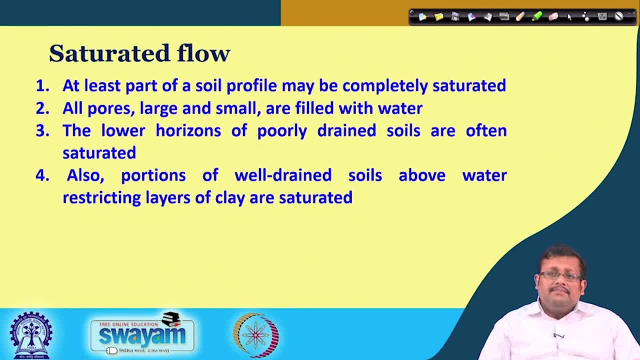 Small pores, both large and small pores- that means macro pores and micro pores- should be filled with, completely filled with water, and the lower horizon of poorly drained soil are often saturated. you must know that and remember that the portions of well drained soils above water restricting layers of clay are also saturated. 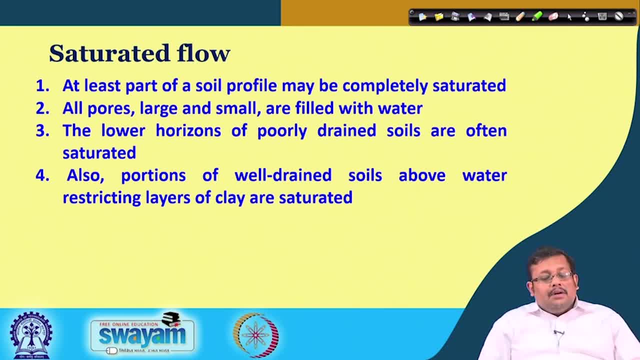 So again, saturated flow occurs. So when you know soil profile is completely saturated, part of the soil profile may be completely saturated and all the pores, both micro pores and macro pores, are filled with water and lower horizon of poorly drain soils are often saturated, whereas the portion of 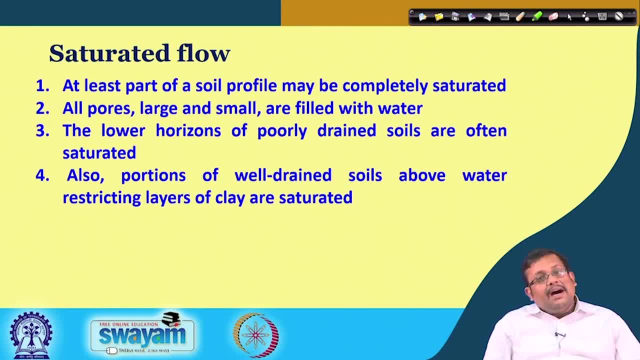 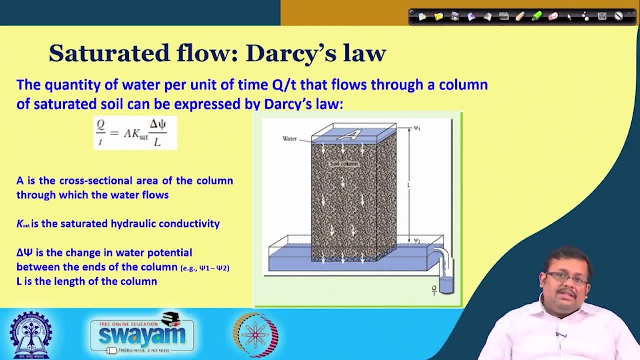 well drained soils above water, restricting layers of clay are also saturated. Now saturated flow occurs, OK, of water within the soil basically obeys a law. We call it Darcy's law. Now the quantity of water according to Darcy's law. let us see the quantity of water per unit of time. 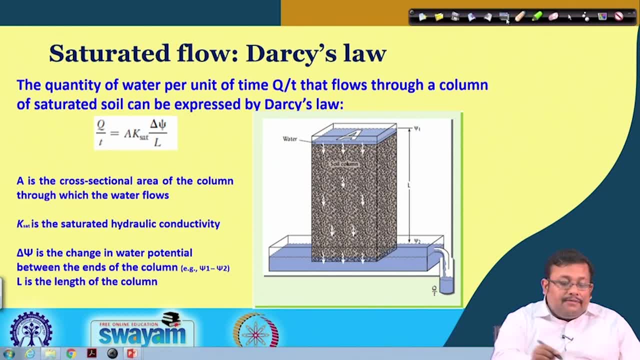 that is, if we denote the quantity of water by q and time as t. So the quantity of water per unit of time, that is, q by t, that flows through a column of saturated soil can be expressed by Darcy's law: that is q by t, equal to A, multiplied by K, sat and multiplied. 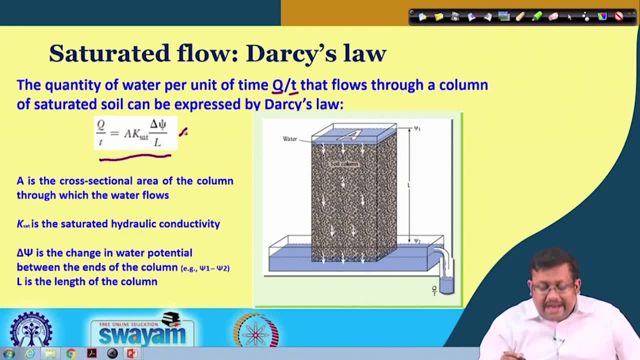 by delta psi over L. Now you see there is a soil column in this picture, ok, And the length of the soil column is L, denoted by L, And the cross section is basically A. this cross sectional area of the water column is A, through which water flows, And the potential at the top of the soil column is psi 1, whereas 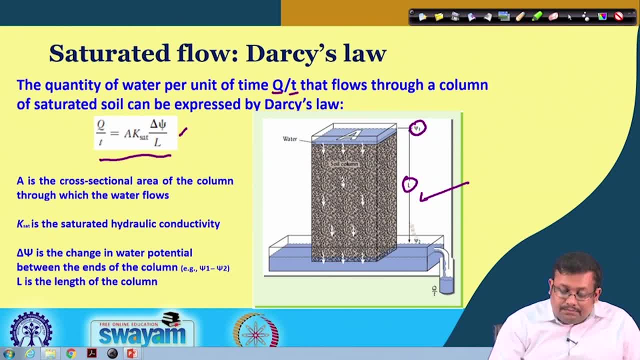 the potential at the bottom of the bottom of the soil column is psi 2.. So, as you can see, water is moving through this soil column and finally it is. we know there is an outlet where water is emitting at a rate of q by t. So here K sat in this. 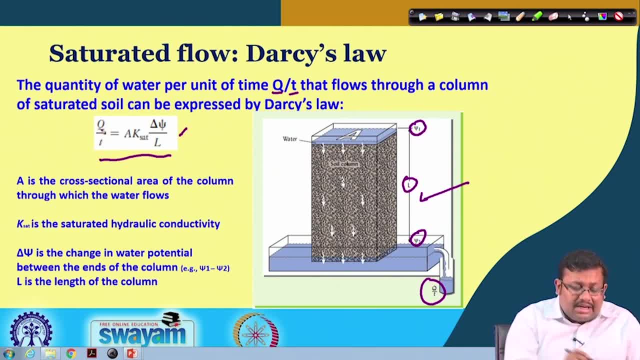 equation K sat. so we already know q is the quantity of water, t is the time. Here A is the cross sectional area, Delta psi is basically the integral area of the soil column, and so this is A here. delta psi: A is the total area of the soil column, So delta psi is basically. 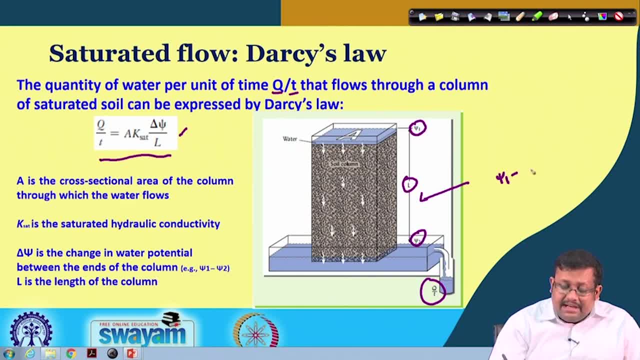 the total area of the soil column, So k sat is the number of hours per hour. that is the difference between potential at the two points. So delta psi is basically the change in water potential between the ends of the column, So, and l is the length of the column, So. 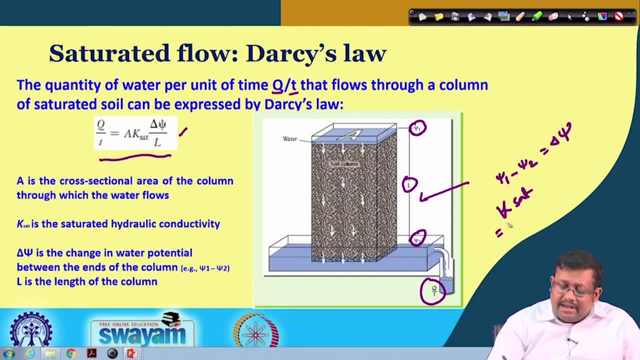 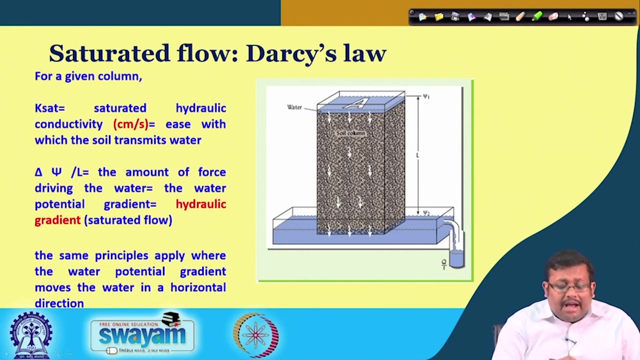 the K sat is basically the saturated hydraulic conductivity. It is very much important for different irrigation and other soil water movement purposes also. we will discuss. So this is called Darcy's law. Let us see what is the implication of saturated hydraulic conductivity. So for a given column, 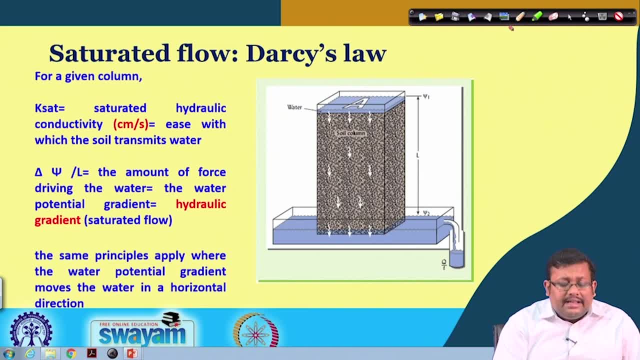 this K sat, or saturated hydraulic conductivity, is expressed in the unit of centimetre per second and basically it denotes the ease with which the soil transmits water. Now, you know this term, that is, delta psi by l. It basically denotes the ease with which the soil transmits water. So the case that 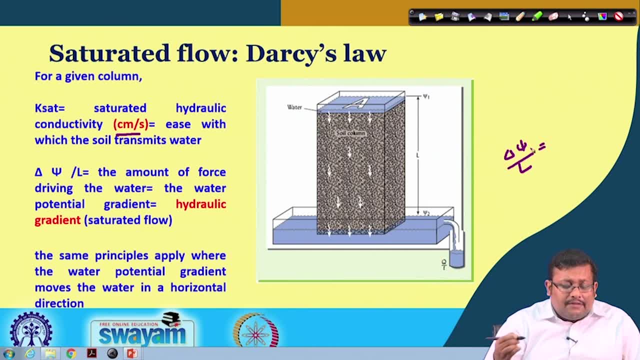 shows the amount of force or the amount of force that driving the water. We call it sometime the water potential gradient and in case of saturated flow it is termed as hydraulic gradient. it is very, very important And remember that these principle of water movement through these, you know, saturated- 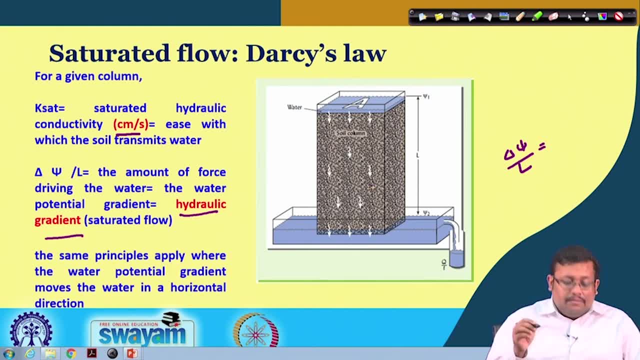 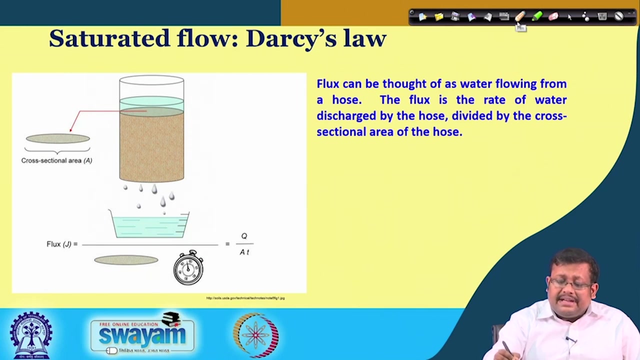 soil columns also. you know also, the same principle also applies with the water. potential gradient moves the water in a horizontal direction. so this is a point to remember. So let us see what is the practical implication Now in case of saturated water flow. this flux, this flux is basically Q by T, Q by T equal. 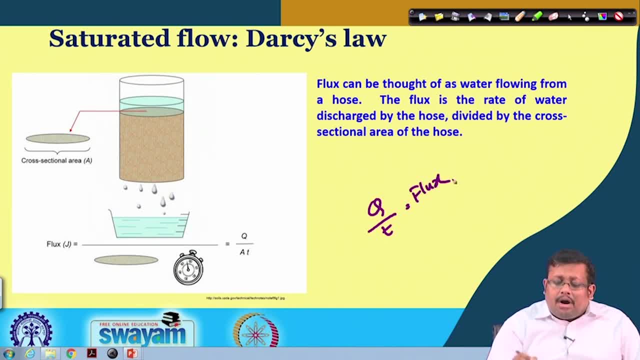 we call it flux of water. Now, this flux can be thought as a water flowing from a hose. when we are watering the garden through a hose, the flux can be thought as a water flowing from that hose. Remember that the flux is the rate at which water is flowing. 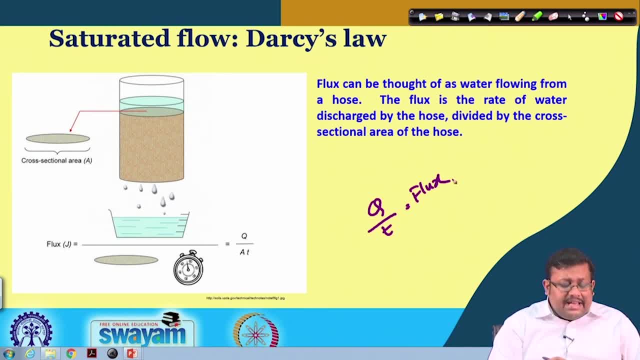 Water is discharged by the hose, which is divided by the cross sectional area of the hose. So flux is basically Q over A into T, So it is the rate of water discharge by the hose, by the cross sectional area of the hose. So this is called the flux. 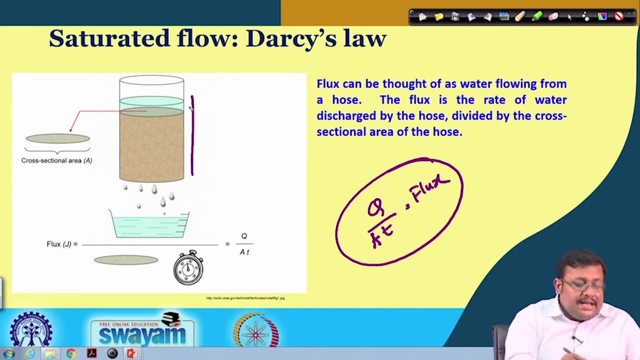 So this is the- if we consider this is a hose, And obviously this is a cross sectional area, A, So flux can be calculated as Q by below, Q by A multiplied by T. So let us see what are the important points to remember in case. 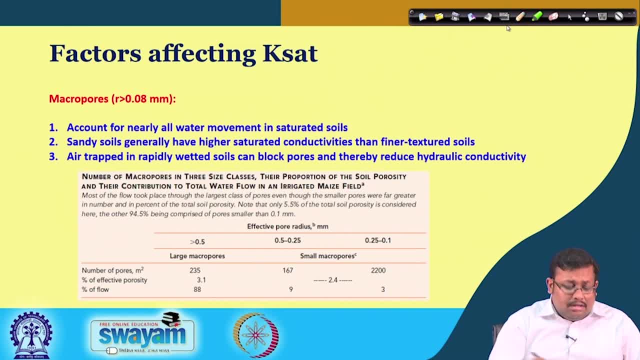 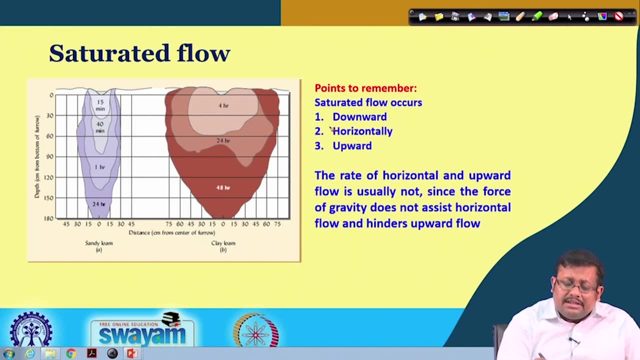 of saturated flow. Remember that. sorry, So remember that in case of saturated flow, Saturation- Saturation, So saturated flow- can occurs both downward, horizontal and upward direction. However, the rate of horizontal and upward flow is usually not similar than that of you. 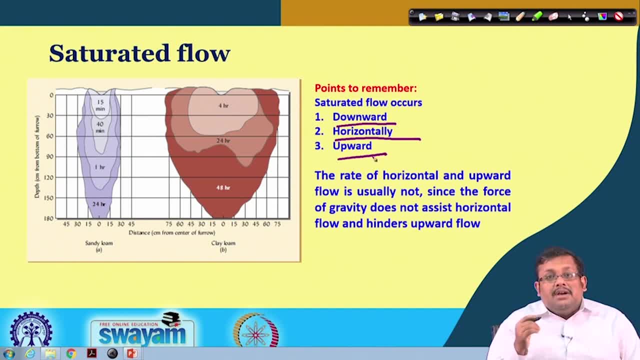 know than that of a downward flow, Because the force of gravity does not assist horizontal flow and also hinders the upward flow. So because of this reason the rate of horizontal and upward flow is not the same, not equal to the rate of downward movement of water through a saturated water. saturated- 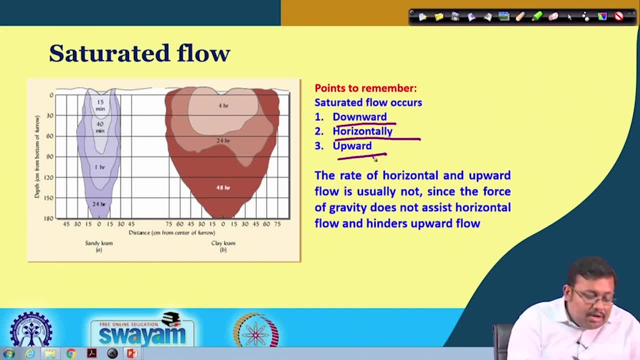 soil column. Now, if you see this picture, I have shown here two example. one is sandy loam soil, another is clayey soil. In case of sandy loam soil, you see the rapid downward movement of water through the saturated- you know, in case of saturated flow. 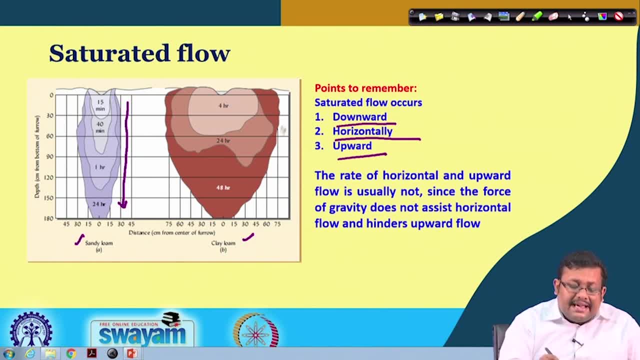 However, these rapidity is quite less in the downward direction. in case of clay loam soil, which is more fine textured soil, However, their horizontal movement is quite high than that of this sandy loam soil, which is coarse textured soil. So depending on the textural classes also the direction of saturated flow also differs. 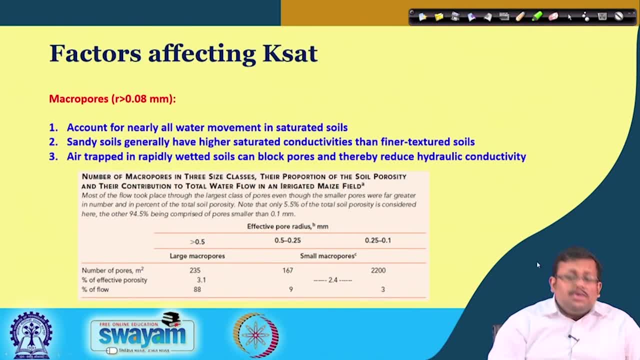 So what are the important factors that affect the saturated hydraulic conductivity? First of all, the macropores. the macropores are, you know, those pores. we have already discussed this macropores. Macropores are those pores which are having a, you know, radius of greater than 0.08 millimeter. 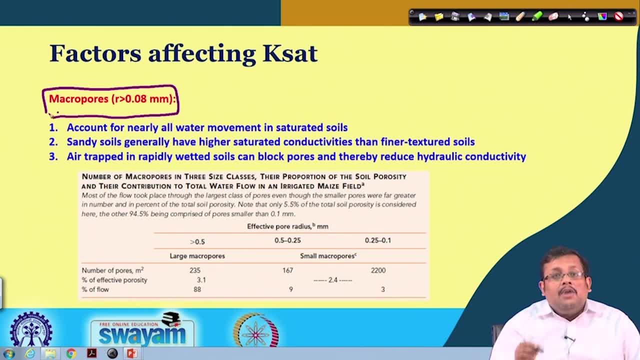 Now, these macropores account for nearly all water movement in saturated soils, And remember that sandy soils you know. so these you know I you know. again, let me tell that these macropores account for nearly all the water movement in case of saturated soil. 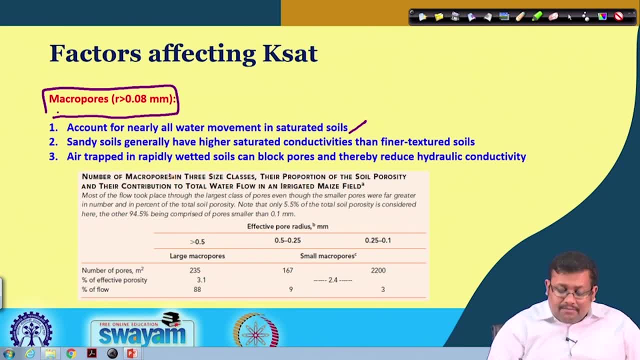 So this can be, you know more, you know- evident from this table where you can see the number of macropores in three slice classes, their proportion of soil porosity and their contribution to total water flow in an irrigated maize field, You can see that 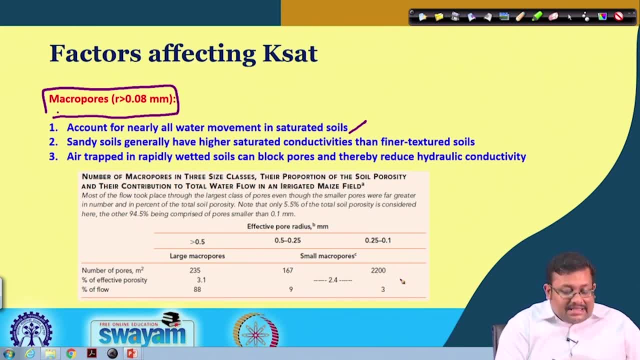 Most of the flow took place through the largest class of pores, that is, large macropores, and there are other smaller pores- we call them small macropores, And you can see percentage of flow: 88 percentage of flow is accounted by this large macropores. 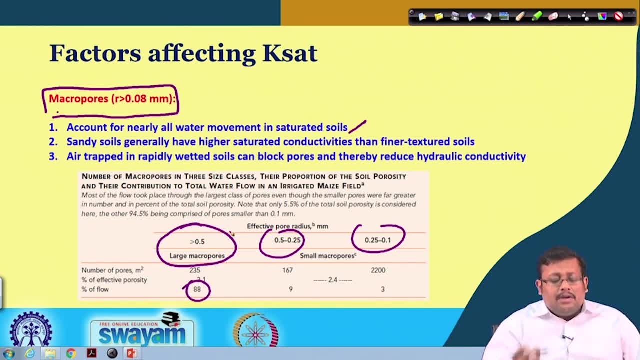 So these results also supports the idea that nearly all water movement in the saturated soil occurs through macropores. Now sandy soil generally have higher saturated conductivity than fine textured soil because obviously in case of sandy soil the number of macropores are quite high. 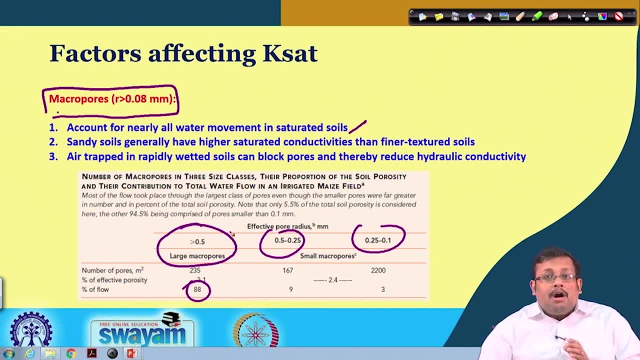 And air trapped in rapidly weighted soil can block pore and thereby reduce the hydraulic conductivity. So this is also very important in case of, you know, macropores. So let us see, So, let us see, So, let us see. 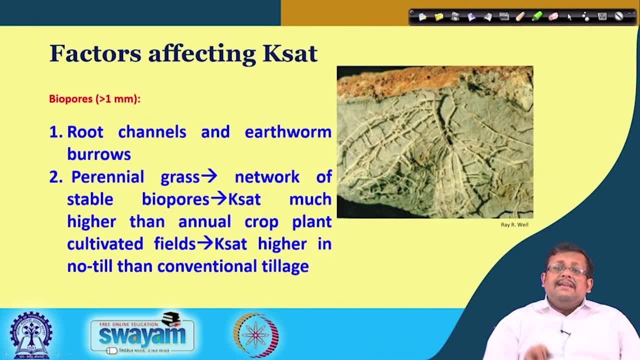 So what are the important aspects? So another important macropore is called biopores. We have already covered biopores in our previous lectures. So another important type of macropores are biopores, and biopores we have already learned. 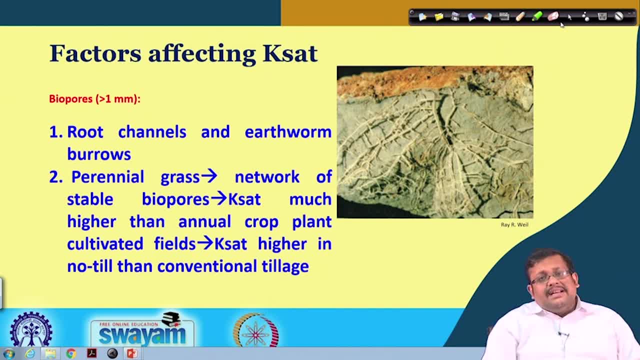 about biopores in our previous lecture. Now, biopores are generally having a radius of greater than 1 millimeter and you know that these biopores are basically root channels and earthworm, you know, created through root channels and earthworm burrows. 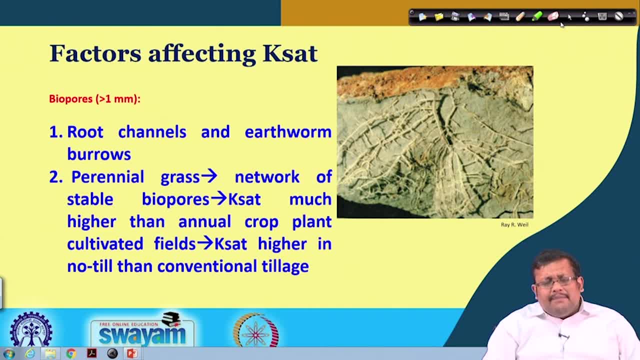 And these biopores help in saturated water flow and also it affects the water. you know saturated, you know water, you know hydraulic conductivity. So if you consider perennial grasses, So if the perennial grasses are responsible for creating a network of stable biopores, 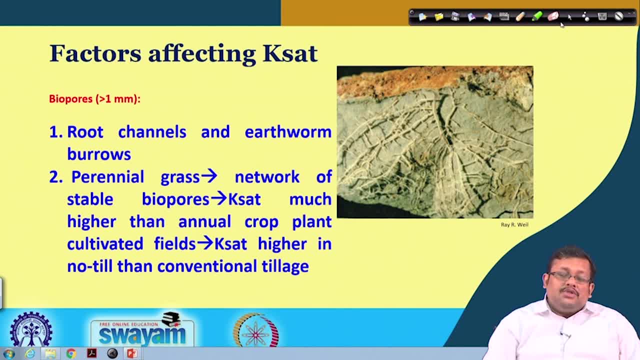 The saturated hydraulic conductivity in case of soil which supports the perennial- you know, which supports the perennial grass- will be much higher than that of soil which is maintained under annual crop plants, Because for growing the annual crop plants you have to uproot all the perennial grasses. 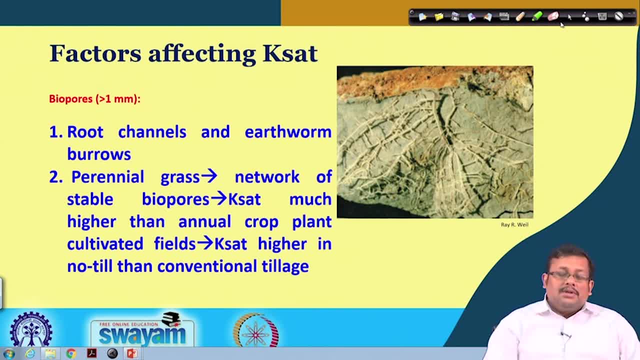 and, as a result, you are breaking down all the biopores also, So the presence of biopores in soil. So once you are breaking down the biopores, obviously the saturated hydraulic conductivity is going further down. So again, in case of soil which is maintained at the perennial grass, the saturated bioconduct. 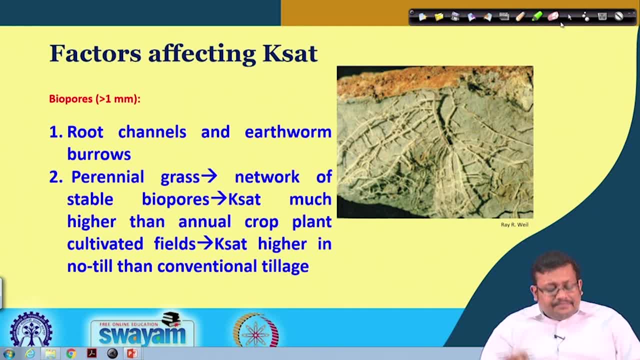 saturated hydraulic conductivity is quite higher than that of, you know, the soil which is cultivated with annual crop plant, And that is the reason that the saturated hydraulic conductivity is higher in low tillage condition than that of conventional tillage. So this is another advantage of using conservation tillage, or in other words, low tillage than 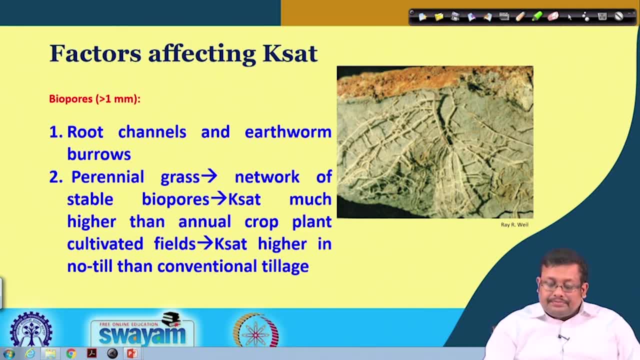 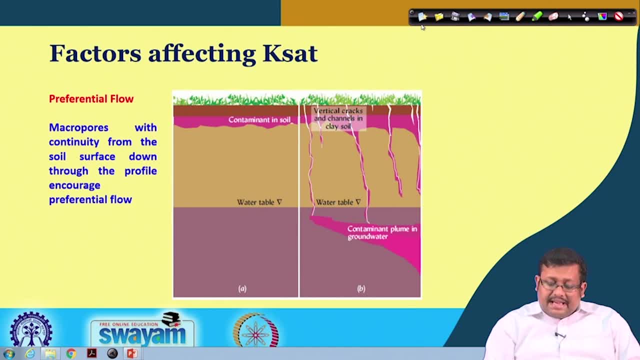 that of conventional tillage. So let us see what are the other factors affecting saturated hydraulic conductivity. So saturated hydraulic conductivity, let us see Saturated. So you know there is another important term called preferential flow. So I have shown here two pictures. 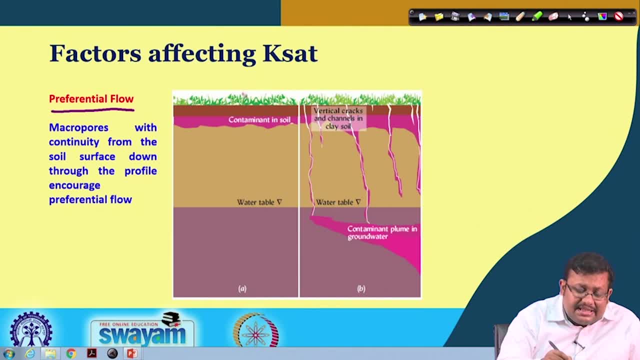 In the first picture. what happened? There is a. you know there is a contaminant, you know there is a deposition of contaminants into the soil, or there is a spillage of contaminant into the soil And it is generally thought that this contaminant will take time to reach into the water table. 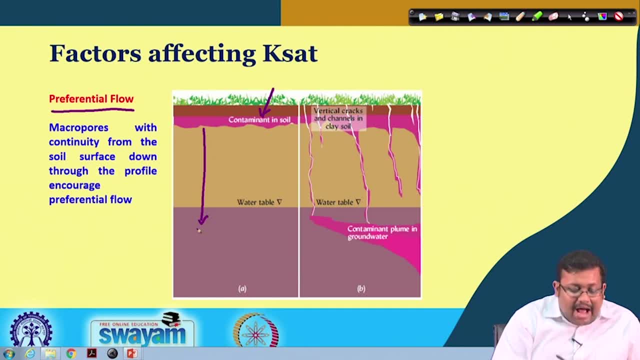 which is far below the soil, However, the macropores. it has been found, after certain period of time, that these contaminants has been already leached or already, you know, already reached the water table and contaminating, you know, and you can see the contaminate plume in the ground water. and these occurs because 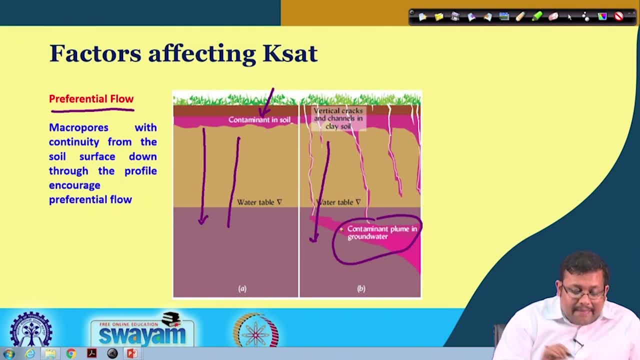 of vertical cracks and channels in the clay soil, So macropores. So macropores with continuity from the soil surface down through the profile encourages the preferential flow. So this is also very important. If there is a flash of rainfall, obviously that will help in movement of contaminant. 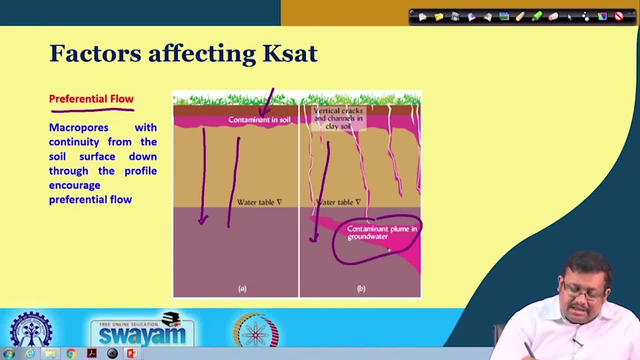 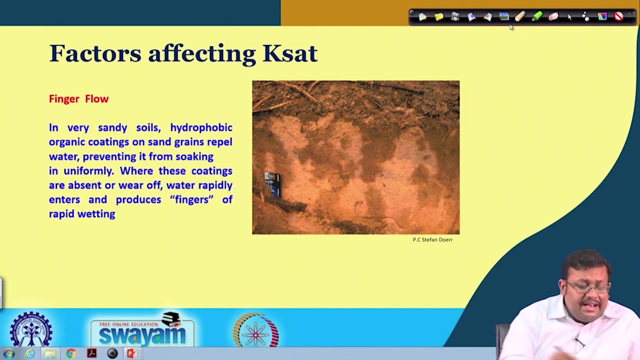 through the soil and ultimately it reaches into the ground water to contaminate the ground water. Preferential flow is very much important, which also affect the saturated- you know, saturated- hydraulic conductivity. Ok, Another important term is called finger flow. Now, finger flow is, as you can see this picture in very sandy soil, hydrophobic organic coatings. 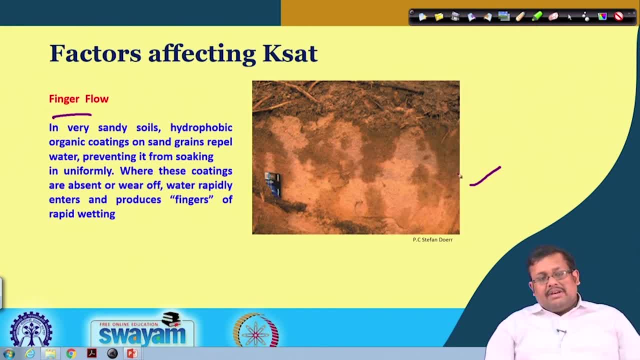 on sand grains repel water because you know when there is a hydrophobic it will repel the water and when there is a hydrophilic it will attract water. So hydrophilic organic coatings are there in case of very sandy soil, with the sand 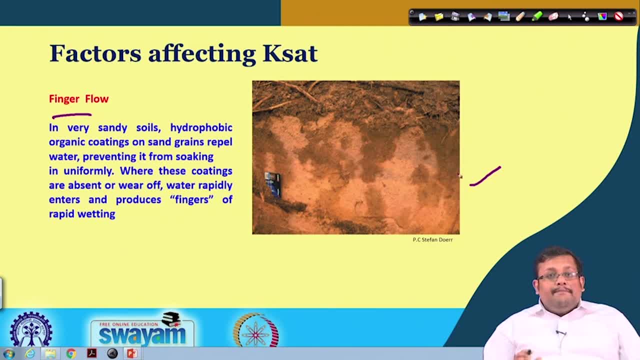 So as a result of this hydrophilic coating, it will prevent the soaking of prevent the prevent the soaking of soil by water uniformly. and where these coatings are absent or wade off, water rapidly enters and produces fingers of rapid wetting. So you can see this picture. 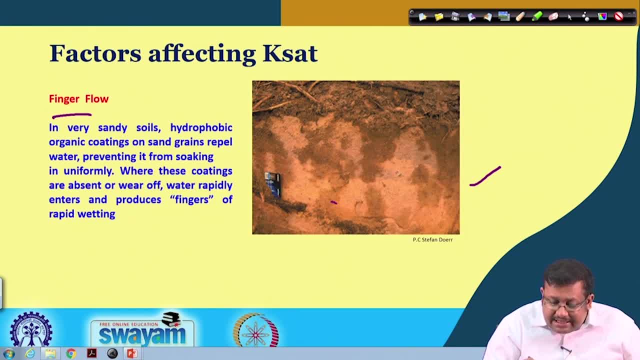 Obviously, this is a very sandy soil, So you can see this picture. So this is a very sandy soil, and this sandy soil may contain some hydrophilic compounds, and these hydrophilic compounds are present in all over the places, and these hydrophilic 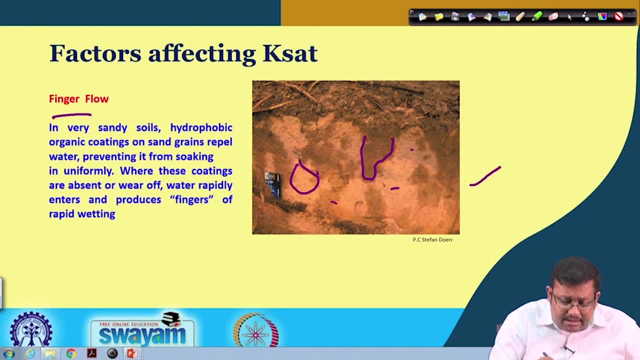 compounds will basically prevent. they may be present here, they may be present here. So all these hydrophilic compounds are prevent basically, or repel the water. repel water, so preventing the from soaking it uniformly, Otherwise it would be, it would have been uniform. 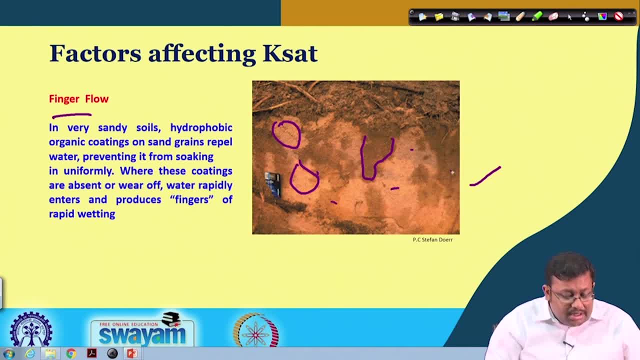 Ok, So where these coatings are absent or wade off, water rapidly enters. So you can see, in this area these coatings are wade off, So water is rapidly moving through this finger like zones. So this is called finger flow of water. 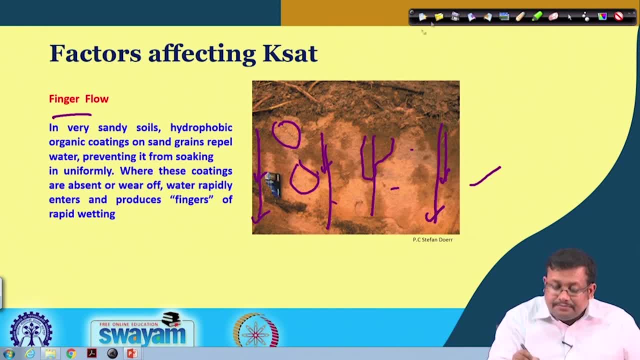 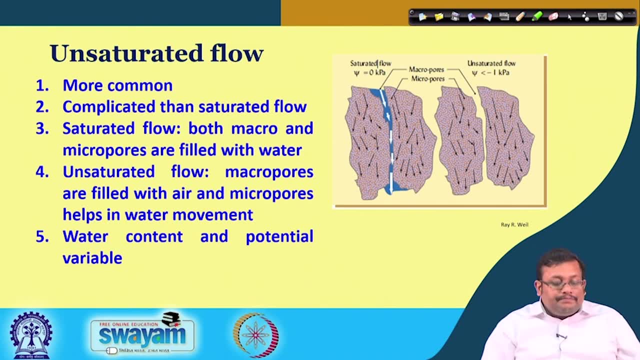 So this also very much important. So let us see about other things, Ok. So let us explore some. Ok, Now, remember that unsaturated flow is more common than that of saturated flow and it is complicated than that of saturated flow. 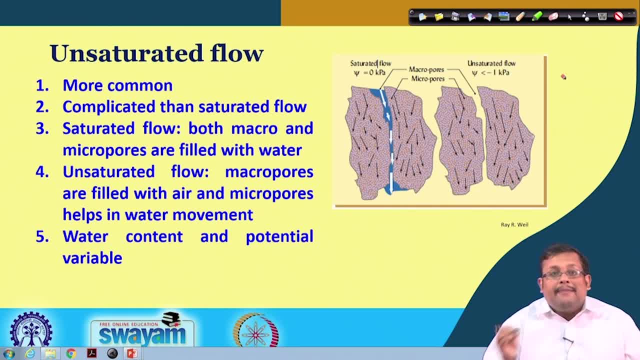 Remember, in case of saturated flow, it occurs when macro pores- both macro pores and micro pores- are filled with water. However, in case of unsaturated flow, macro pores are filled with air and micro pore cells in water movement. And remember that these, in case of unsaturated flow, the water content and potential are very 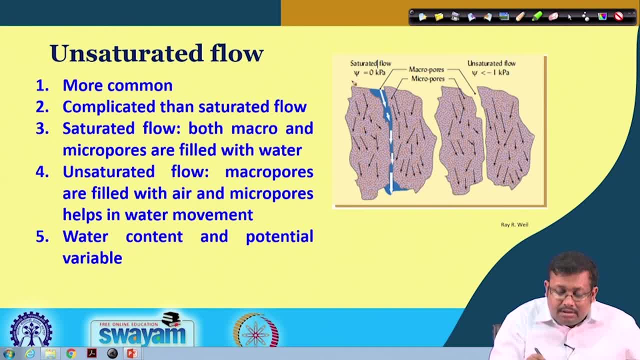 heavy. So, as you can see, in case of saturated flow the potential is 0.. So the both the macro pores and micro pores are filled with water and in case of unsaturated flow, when there is a less or negative potential, all the macro pores will be drained and only. 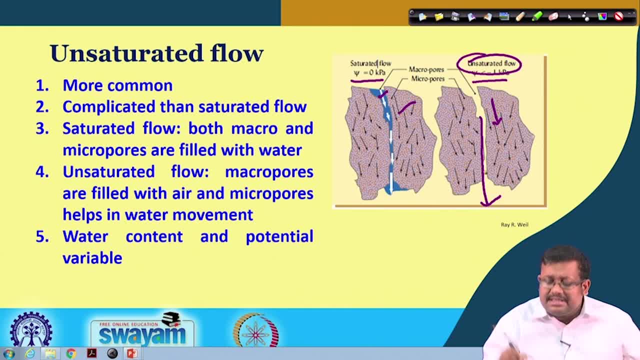 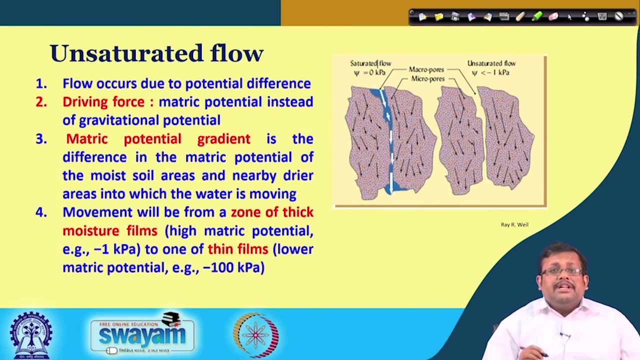 the water will flow through these micro pores. So this is that example of unsaturated flow and this is very important from the point of view of soil water movement. So this unsaturated flow occurs due to potential difference and in case of unsaturated flow, 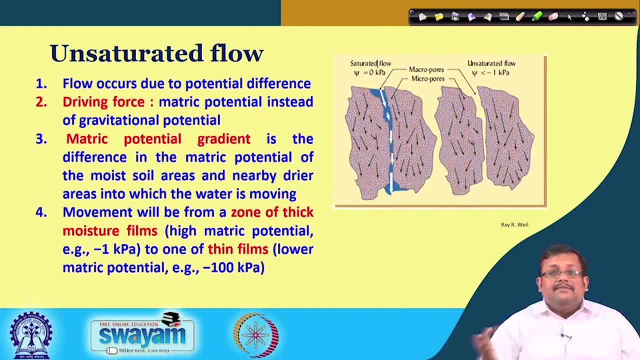 remember, the driving force is the metric potential instead of gravitational potential. So, in case of unsaturated flow- you remember that we are calculating this- you know hydraulic gradient, where this length is, you know, very much important. However, in case of unsaturated flow, this will not be the case. 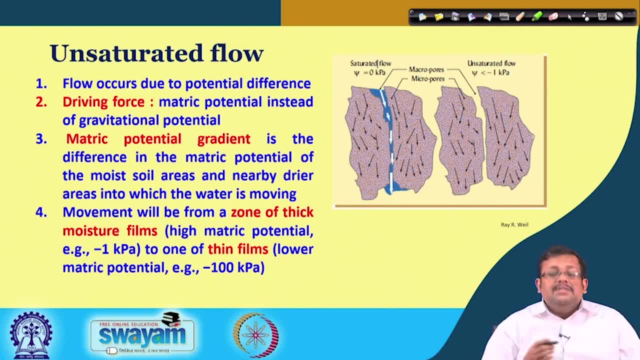 All right, Thank you. flow: this metric potential is very much important than that of a gravitational potential. And metric potential gradient is the difference in the metric potential of the moist soil areas and nearby dry areas into which the water is moving. So water will always move from higher metric potential to lower metric potential. 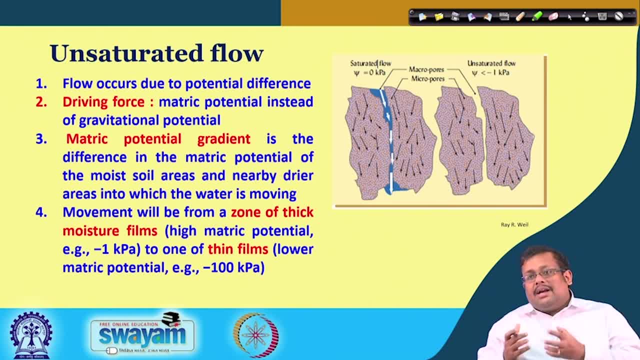 Lower metric potential means the attraction for water from the soil matrix is quite high. So water will move from higher metric potential to lower metric potential areas in case of unsaturated flow, And movement will be from a zone of thick moisture film- obviously higher metric potential. 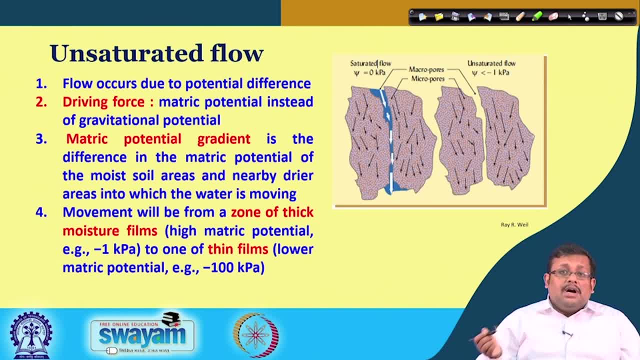 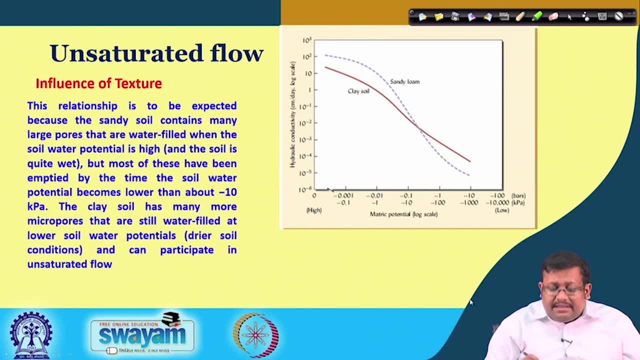 example, minus 1 kilo Pascal to one thin films to one of thin films. that is lower metric potential, that is minus 100 kilo Pascal. So this slide shows the influence of texture. as you can see, we have plotted here the metric potential in the log scale in the x axis. 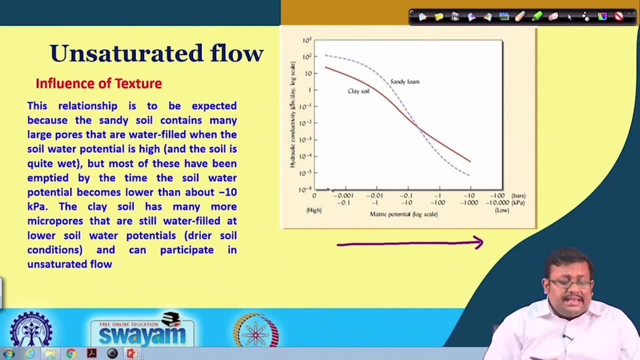 And the y axis there is a hydraulic conductivity. so you can see that there is relationship, is to be expected because you can see at higher metric potential, or I would say at higher metric potential means high water content. obviously the hydraulic conductivity is quite high in case of sandy soil than that of a clayey soil and the trade you know alters. 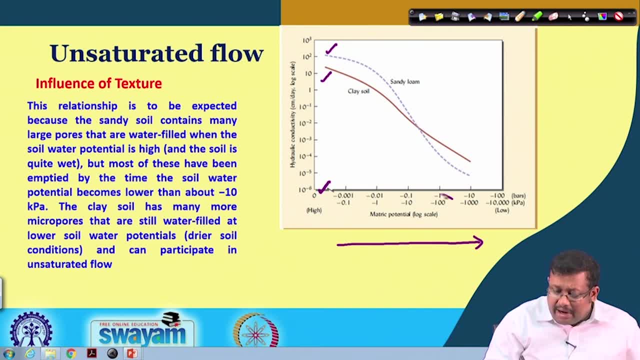 and the trade reverse when the metric potential is higher. So this slide shows the influence of texture. So the metric potential is quite low, that is, low moisture content. So this relationship is to be means quite, you know, expected because it is sandy soil. 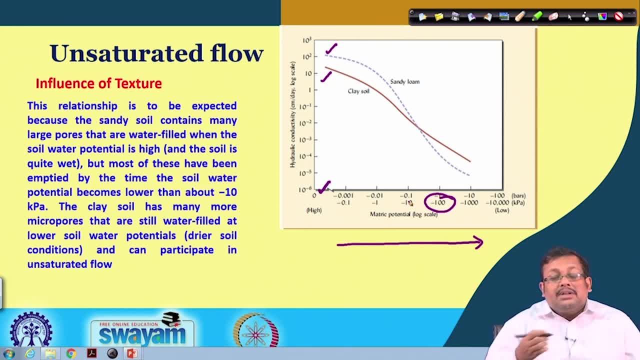 contains very large pores that are water filled. when the soil water potential is high and the soil is quite wet, But most of these have been emptied by the time, the soil water potential becomes lower. that means in this zone. So when the soil water potential lower down from 0 to minus 100 kilo Pascal, then the 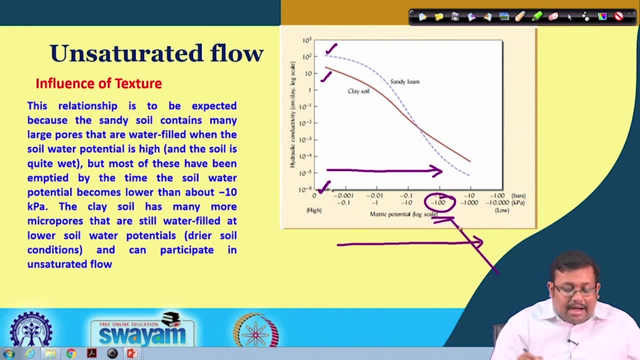 soil water potential becomes lower. So when the soil water potential is not 100 kilo Pascal, obviously you know these larger macro pores will emptied first, leaving only the micro pores which are present in clayey soil. So the clayey soil has many more micro pores that are still water filled at lower water. 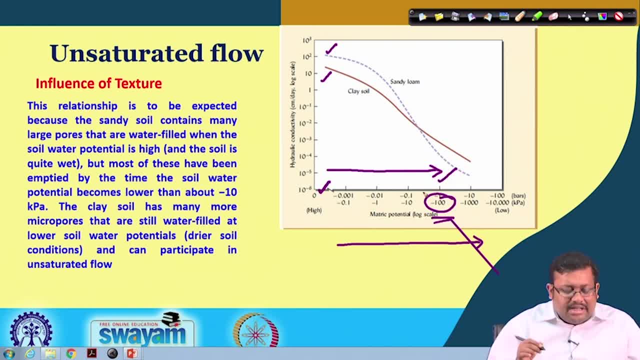 potential at this point. So in the drier soil condition and in this condition they can participate in the unsaturated flow. So you can see, at at lower metric potential, or in other words, in lower water potential, they can participate in the unsaturated flow. 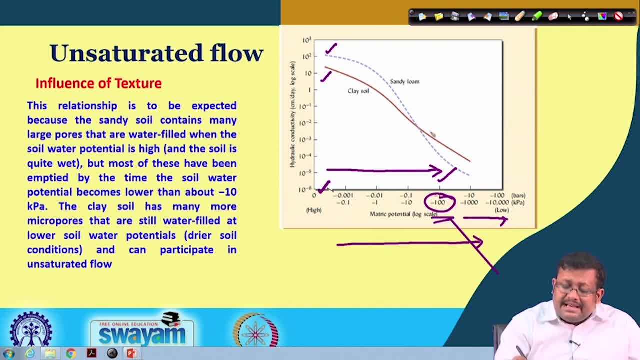 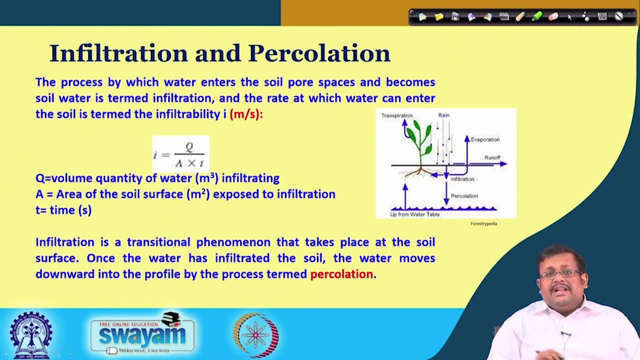 moisture content. these clay soil are taking part. you know are mostly important for unsaturated flow of soil water. Another important term is infiltration and percolation. Now, infiltration is the process by which water enters in. the water enters the soil pore space and become soil water, and the rate at which the water can enter into the soil is termed. 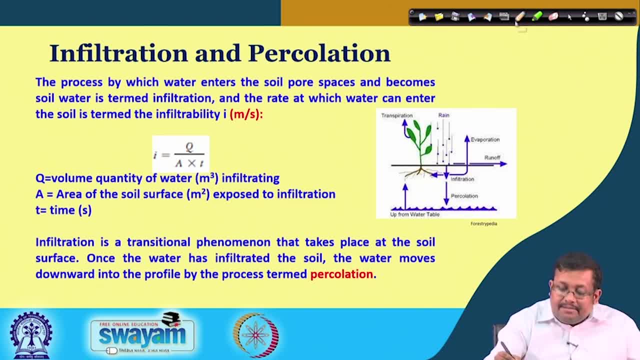 as infiltrability, and we generally term this as small i and remember the form. the unit of infiltrability is meter per second, So infiltrability is basically expressed in these terms. So i equal to q over a into t, where q is the volume of quantity. volume and quantity. 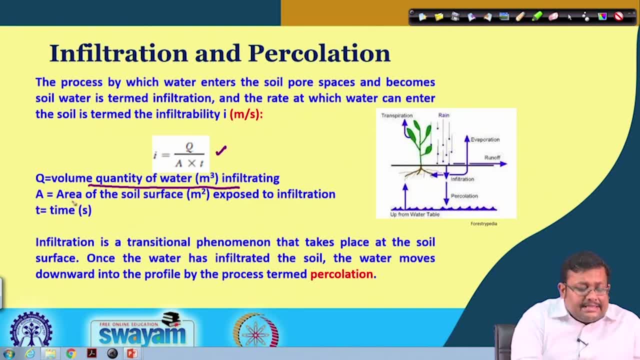 of water in cubic meters. A is the area of the soil surface in square meter exposed to infiltration and t is time in second. So infiltration is a transitional phenomena. remember that infiltration is a transitional phenomena that takes place at the soil surface and remember that was the water has infiltrated. 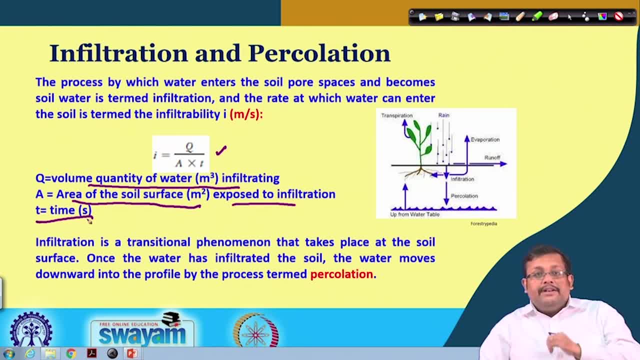 into the soil. the soil water moves down downward into the profile by the process termed as percolation. So you can see this picture. this is the soil surface. So when there is an infiltration, obviously it will be a surface phenomena- water will enter into the soil and once water will enter into the soil it will move down to the soil. 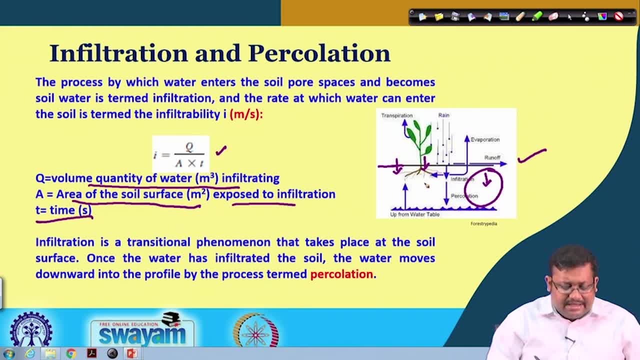 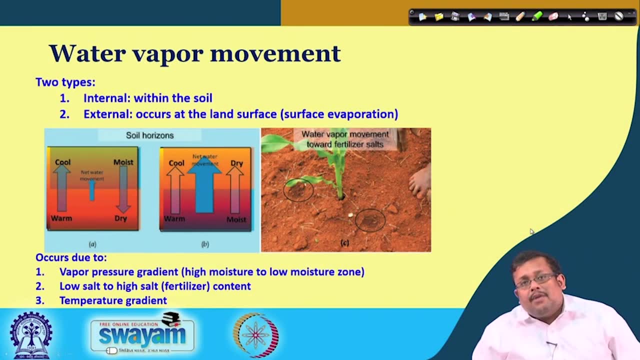 profile, and these movement of water in the soil profile is termed as percolation. it is also very much important, and So this is the difference between percolation and infiltration. The last type of water movement is called water vapour movement, And water vapour movement can be of two types. one is internal, which occurs within the soil. 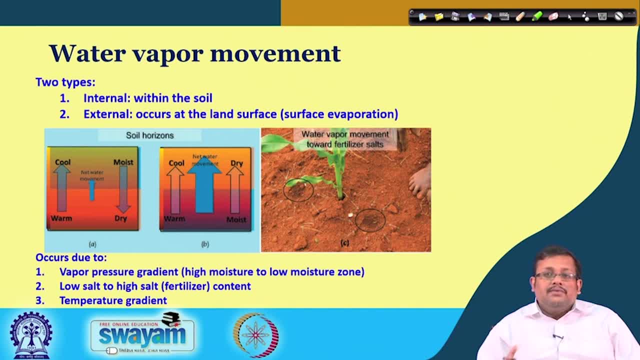 another is external, which occurs at the land surface, or we call it surface evaporation also. So the water vapour movement basically occurs due to three major driving force. The first one is vapour pressure gradient. that is, vapour pressure gradient. that means the vapour will move from the higher moisture to lower moisture zone. 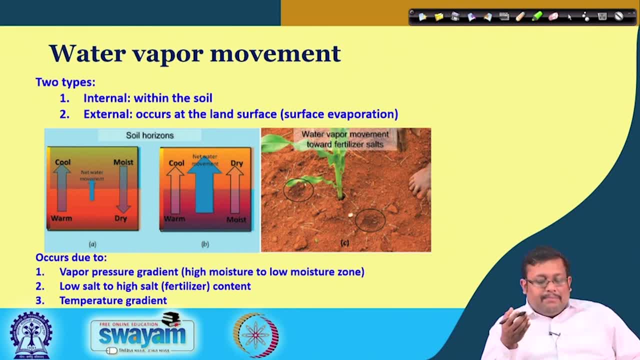 Obviously, When the moisture content is high, obviously the vapour pressure will be high, and when the moisture content is low, vapour pressure also will be low. So vapour will always move from higher moisture content zone to lower moisture, low moisture zone within a soil and low soil to high soil content and low soil to high soil content. 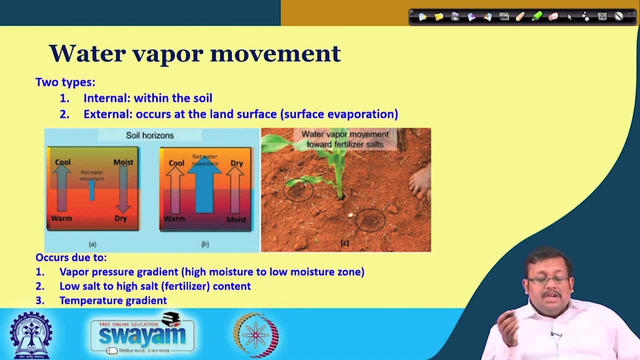 or in other words, it is low fertiliser to high fertilizer content, because where there will be low fertiliser content, there will be higher vapour pressure, as compared to when there is rain. Okay will be high fertilizer content, there will be low vapor pressure. 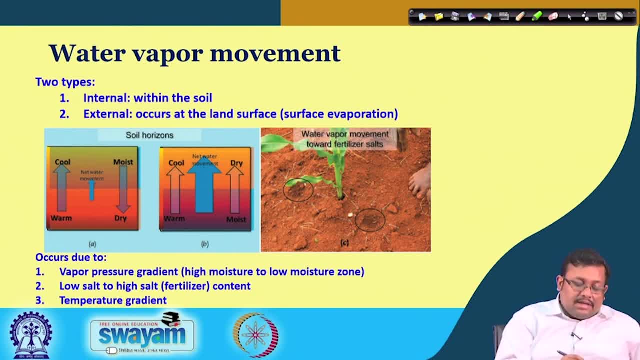 So water will move from low salt or fertilizer content to high salt or fertilizer content. And thirdly is water will always move from according to, along with the temperature gradient, that is, from high temperature zone to low temperature zone. So you can see this picture also. it has been evident. 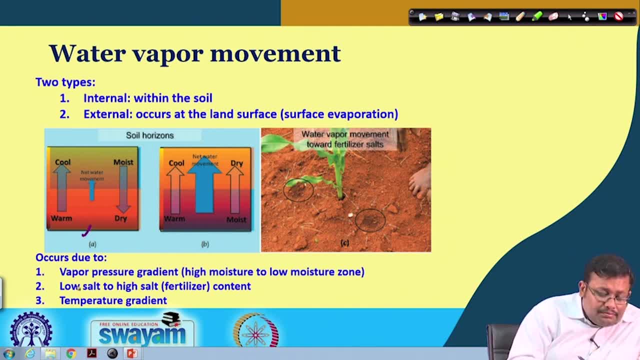 So in this first picture, you know, net water movement is basically nullified by, you know opposite direction of this temperature gradient and moisture gradient. And here the net water movement is quite high because in both the- you know- temperature gradient as well as moisture gradient acting in a same direction.